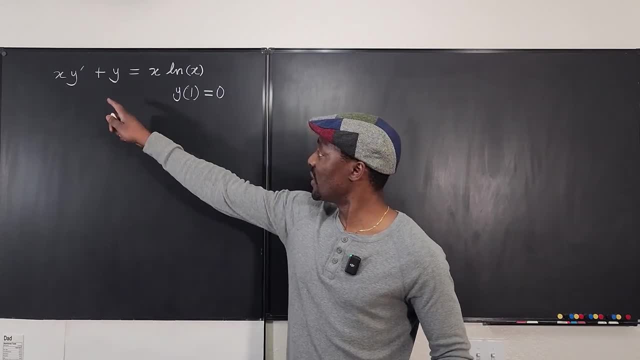 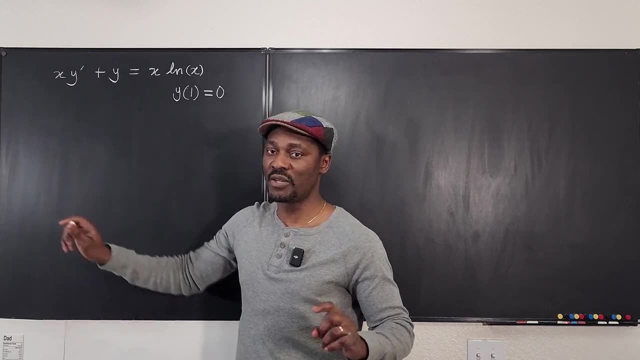 practice you want to do every time you see a differential equation. But looking at this, I know that the only Y that was differentiated, it was differentiated once. So it's a first order differential equation, but I don't know if it's separable or not. Is it linear? Well, 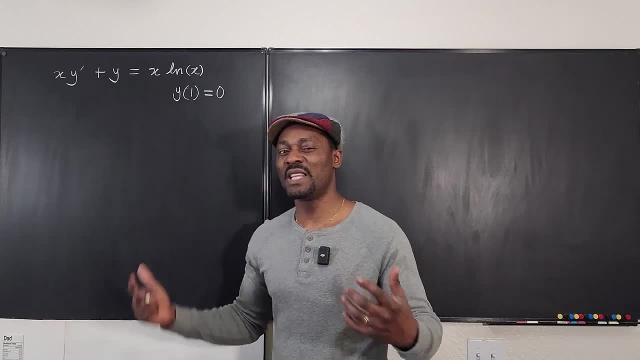 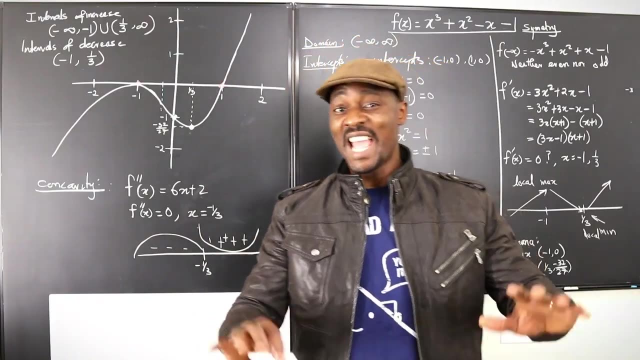 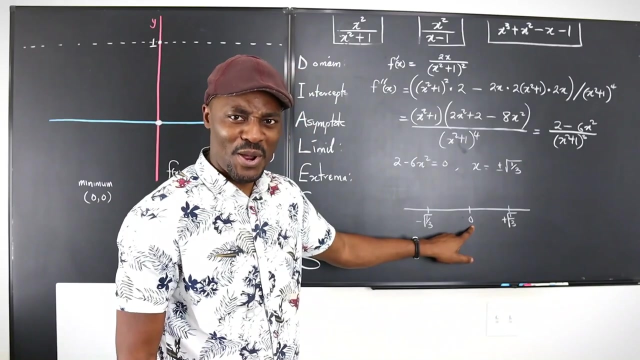 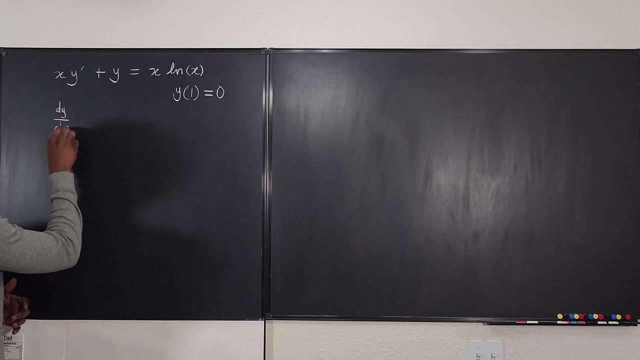 we have to try to write it in the standard form and see if we can get it to look like what I'm about to show you. You're going to have dy dx will be equal to or no to be, dy dx plus p of x times y. 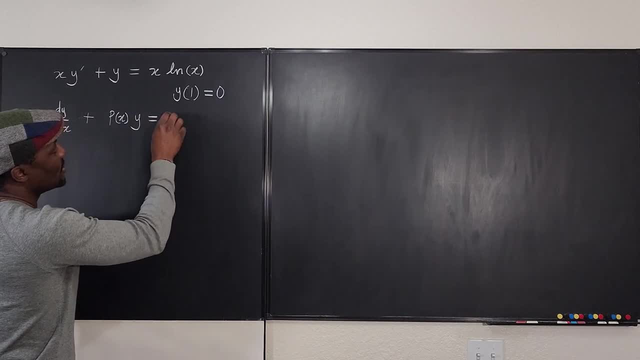 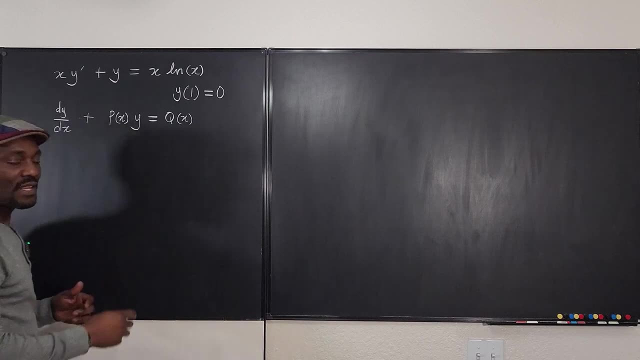 And on the right hand side, you're going to get a function which we could write as: let's write it as: q of x. Now, if you can make this look like this, you're going to get a function. then it is a linear differential equation, a first order differential equation in the 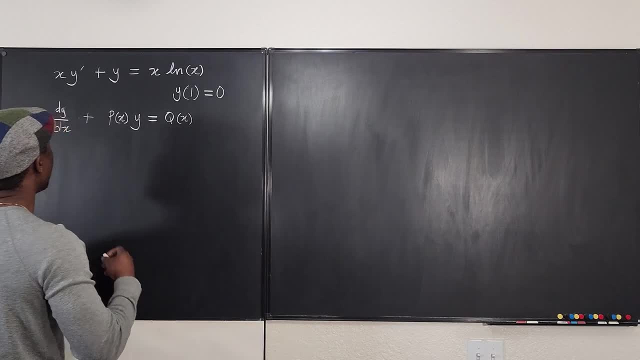 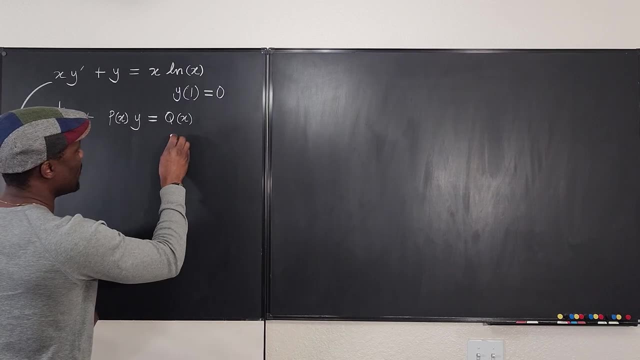 standard form. So let's see if we can do that. Now I'm going to rewrite this y prime as dy dx, So I'm going to have. let's bring this down here. So we're going to have. so this is the standard form, don't forget- And this is our initial condition, It's going to help. 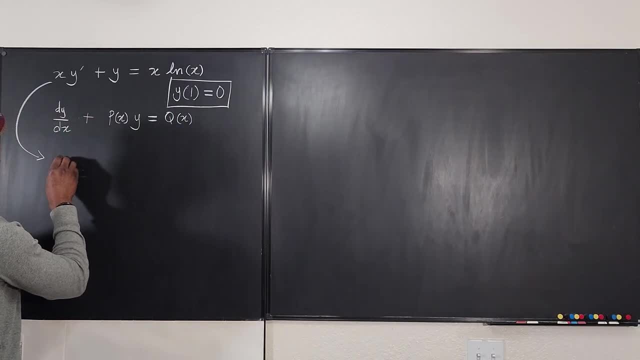 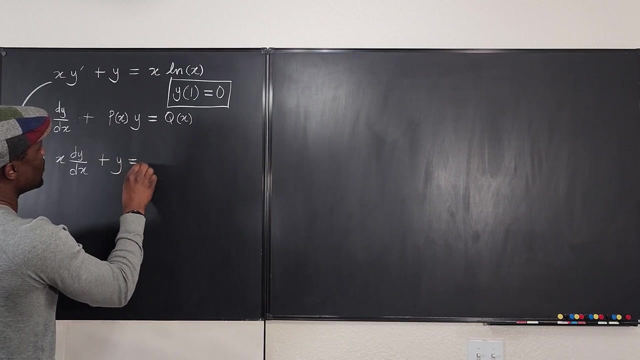 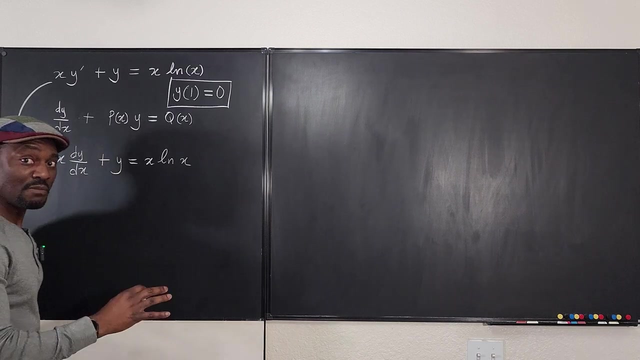 us find the constant at the end. So we have x multiplied by dy dx And we're going to have x plus. you have just y equals x, natural log of x. Now let's see, we need this guy to stand alone and it's the most important thing to do first. So I'm going to divide. 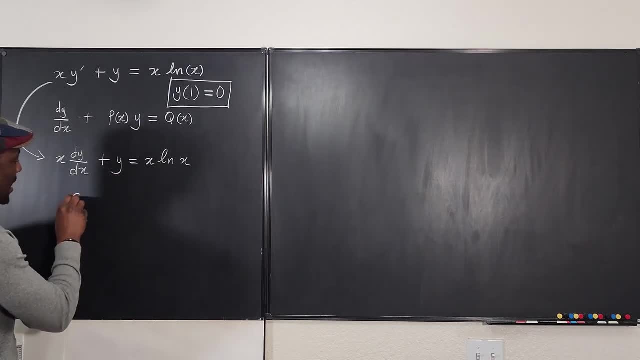 every term by x. And if I divide every term by x, I'm going to end up with dy. dx is equal to sorry, not equal to plus. Well, if this divides this, is going to be one over x times y. And if I divide this by: 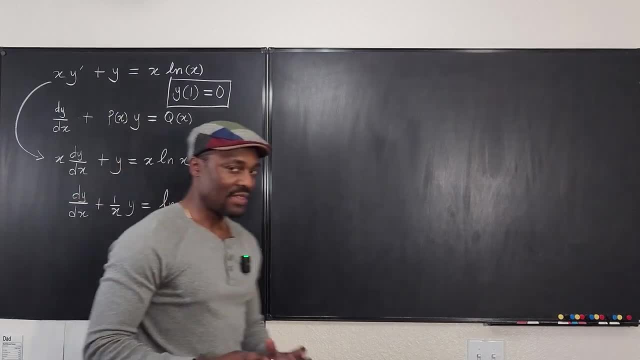 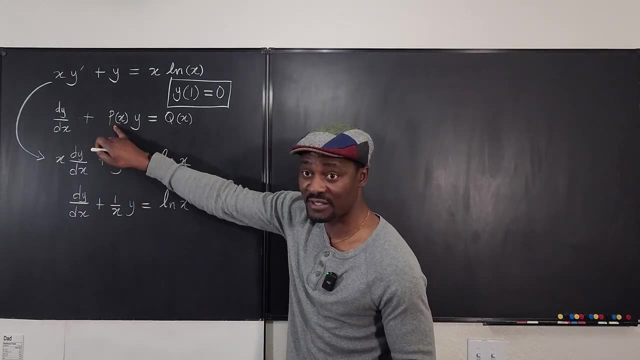 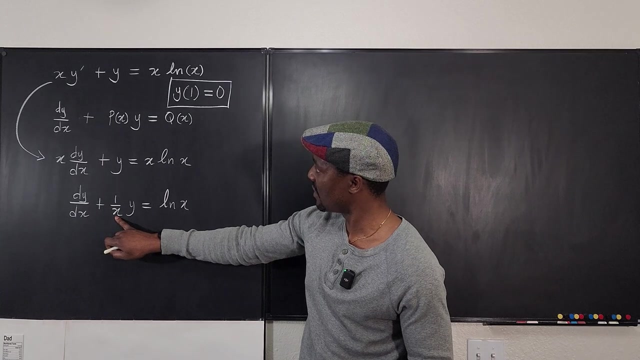 x. I get natural log of x. At this point it looks like what I have here, looks like this: I just need to identify what my p of x is, because that's what I need for my integrating factor. So if I look at this, my p of x is one over x. Okay, so we can say that p of 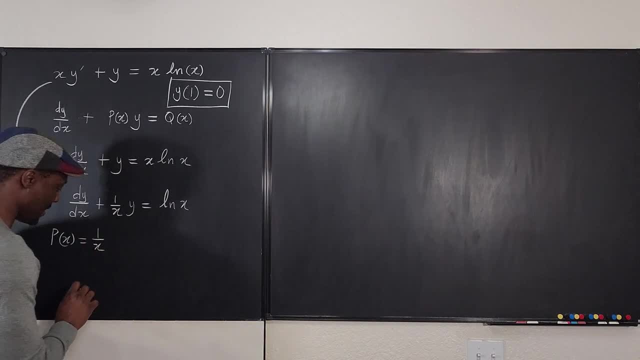 x is one over x. therefore, the integrating factor which you must always get when you have this in standard form, is equal to e, to the integral of p of x. Okay, and in this case it's going to be: let's see, we can actually do it here, It's going. 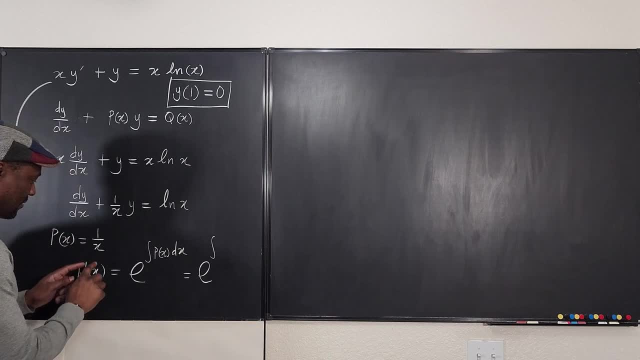 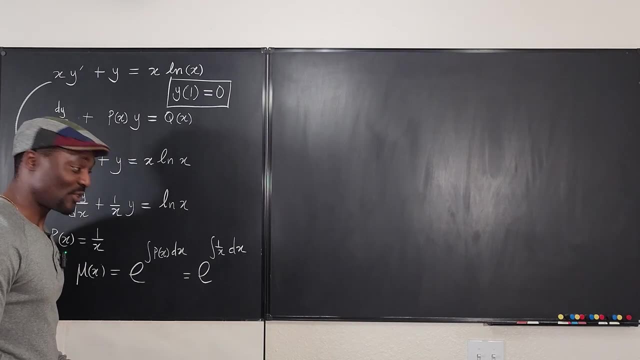 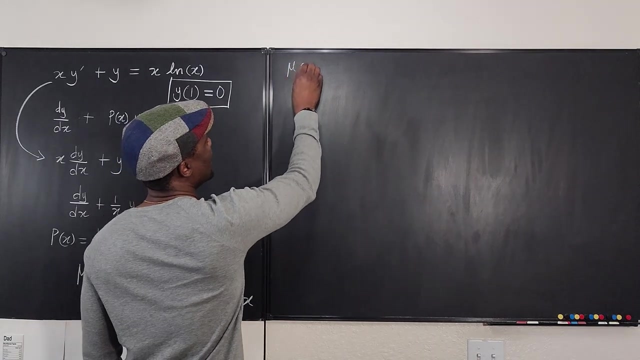 to be e to the integral of what is our p of x, one over xd, x. what is the integral of one over x? It's natural log of x. So this is the same thing as e to the ln of x, which is x, Because this will cancel this out and you have x. so our integrating factor is x. so we can say that the 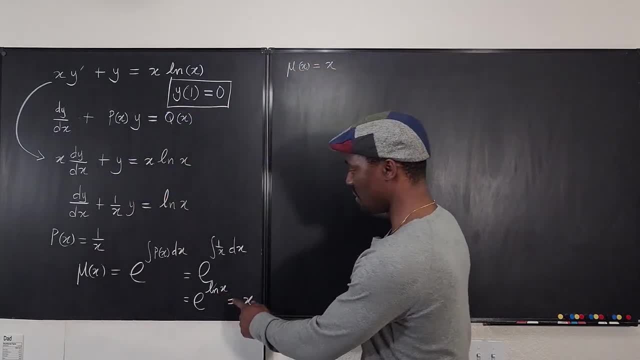 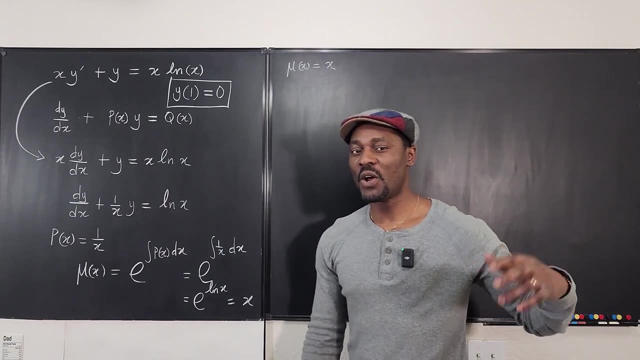 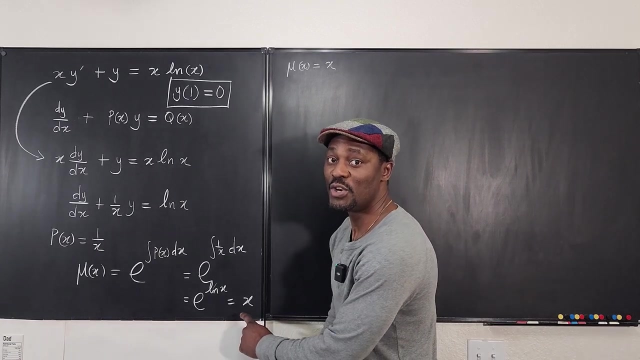 Integrating factor is x. that's the most work you're going to do at the beginning of your setup And once this is done, you want to do this. I Showed this in other videos, but I will no longer spend time showing it. the point of getting the integrating factor is because you know that. 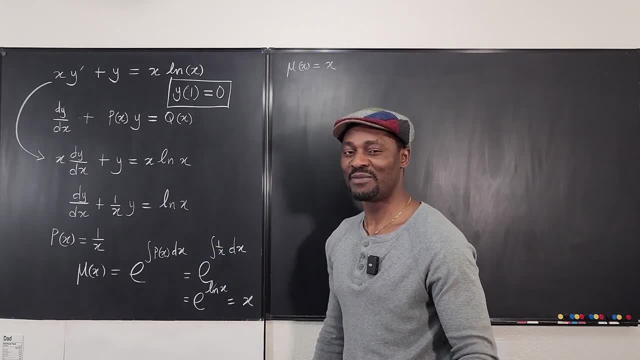 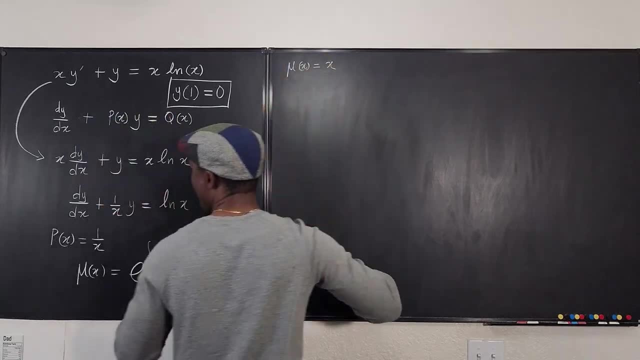 Maybe I should show it, in case this is the first time you're watching a differential equation video using integrating factor, So let me just show it. so you use this x now, you take this x and you multiply every term. That is in the standard form. remember, This is the standard form we generated, okay. 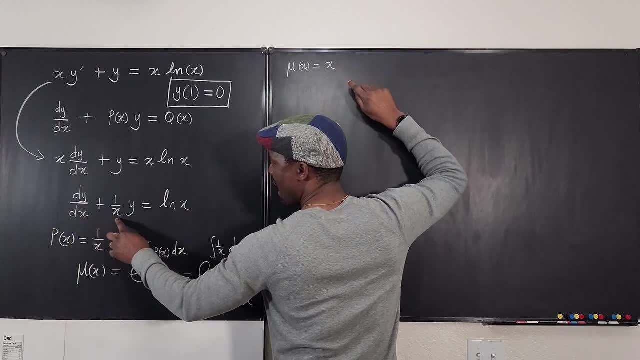 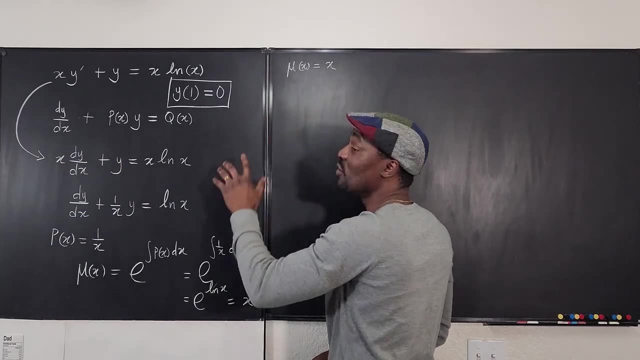 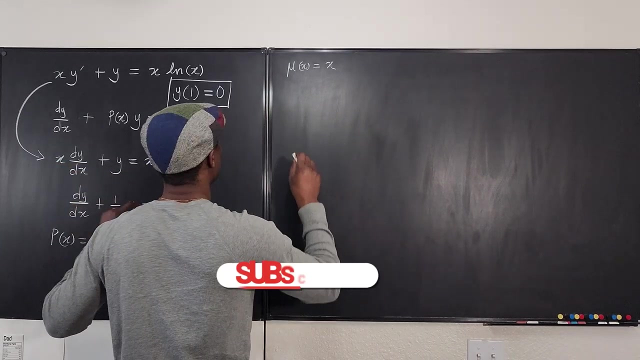 So multiply this by x. multiply this by x. Okay, I know we divided by x before, but sometimes you don't get. most times You don't get the same answer as what you used to divide. So let's multiply it back again and see what we get. so if we multiply again, We're going to get x. 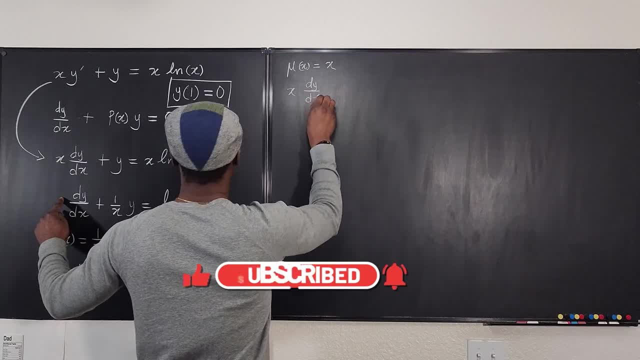 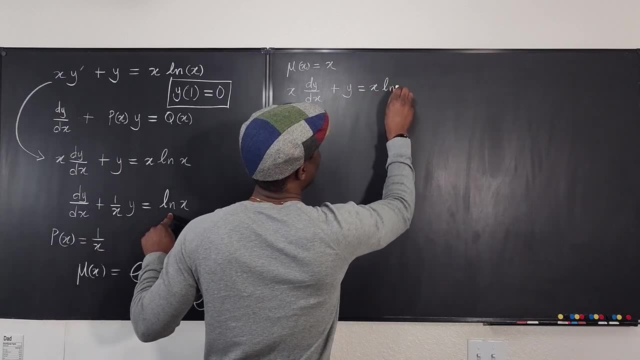 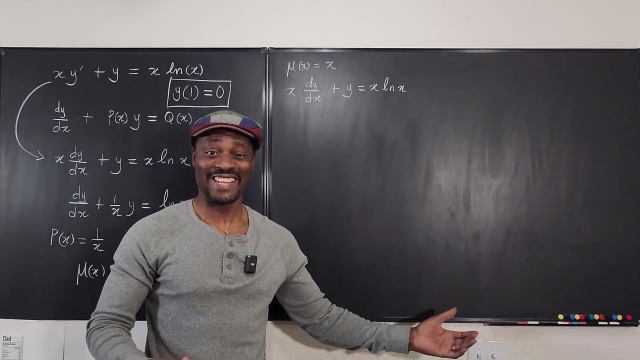 times dy, dx, For multiply this by x, we're going to get just y, and if we multiply this by x, we get x, ln, x. So this equation was already in the form. that was easy, but I I Didn't see it. Okay so, but if you saw, it is just still better that you show your work. 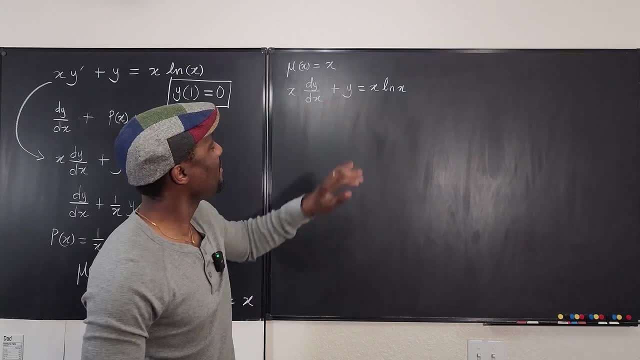 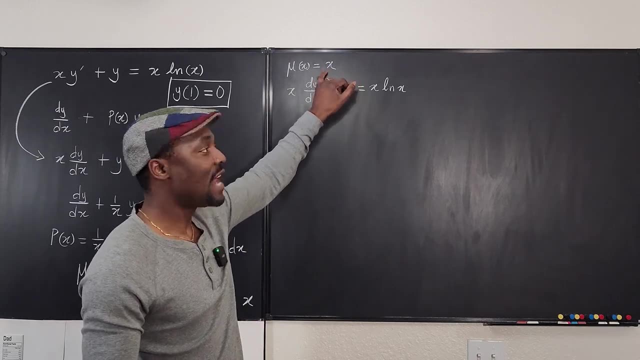 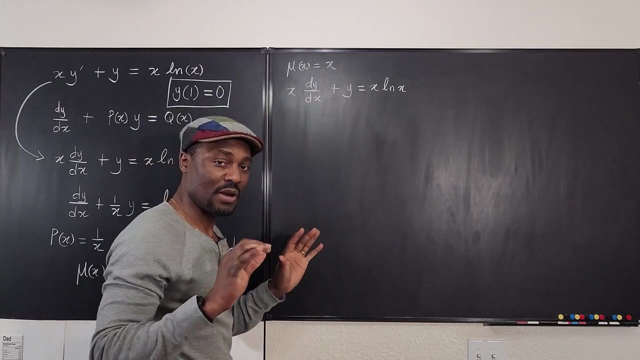 So you're sure that what you're doing is correct. So now I have this. now, What does this mean? Automatically, whenever you're you get your integrating factor and you use it to multiply Everything, the left hand side automatically becomes the product, just the product. Okay, Let's do it this way, look. 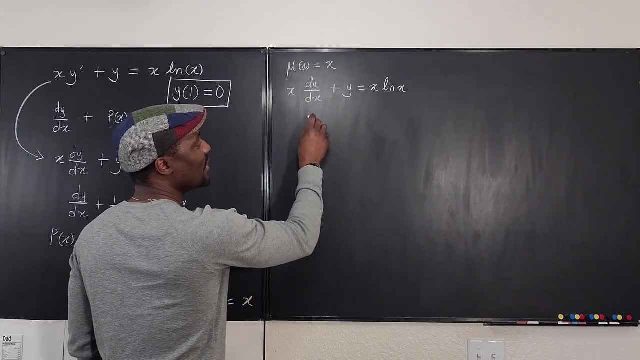 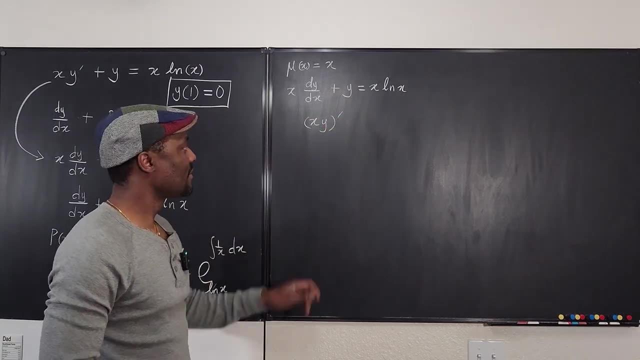 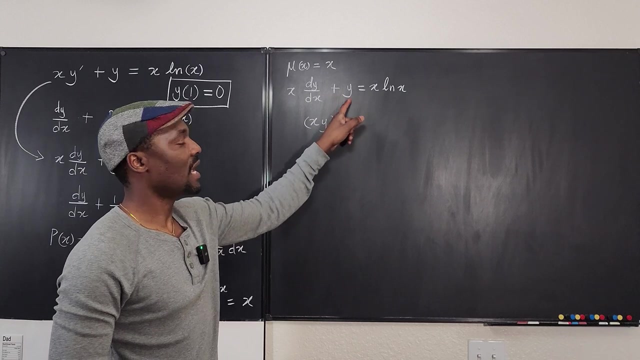 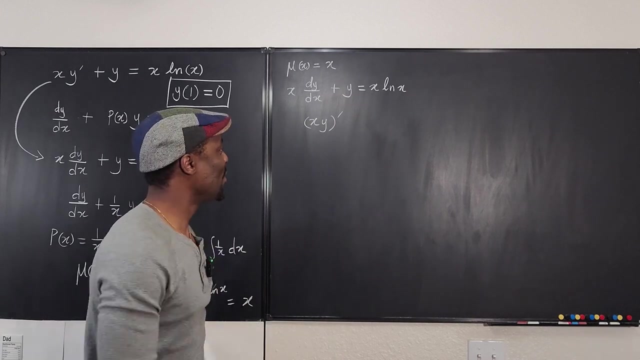 This looks like we have applied the product rule to the derivative of xy: Keep the first, differentiate the second, Differentiate the first, keep the second. do you see that? so this expression looks like the derivative of x times y. Okay, so we're going to keep the left hand side. So this is what we have. natural log of x. 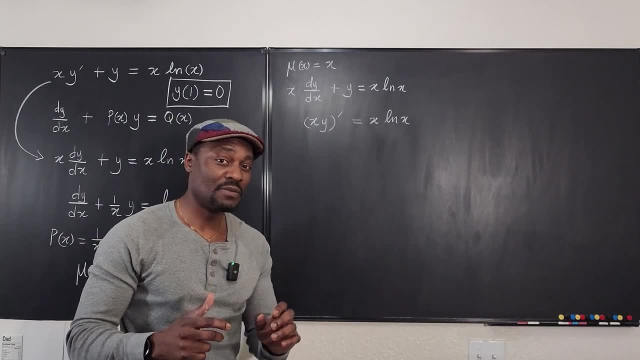 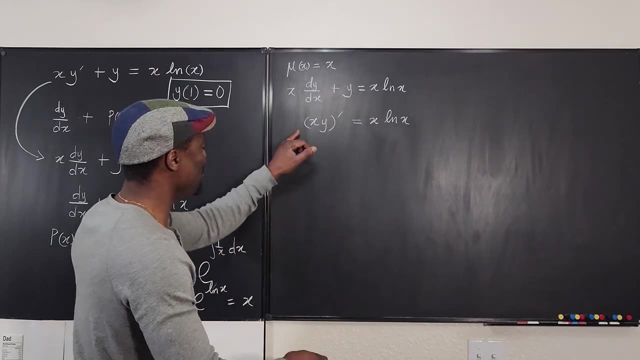 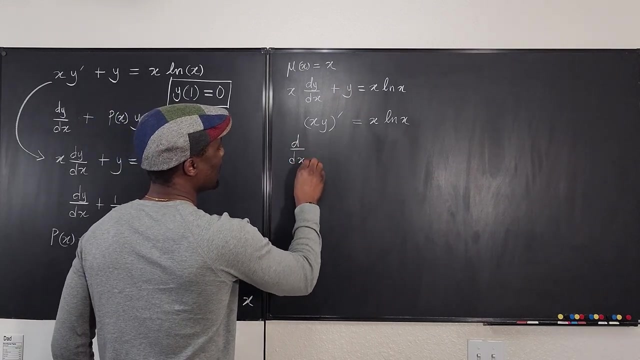 So let's solve it. Remember, our job is to find y. that's the point of solving a differential equation: You're looking for the function that was originally differentiated. So now, what does this mean? This looks like we took the derivative ddx of xy. 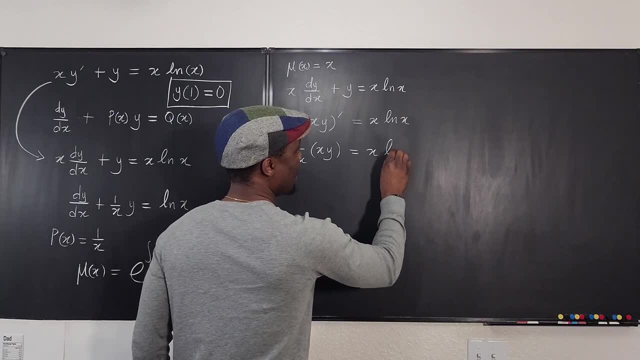 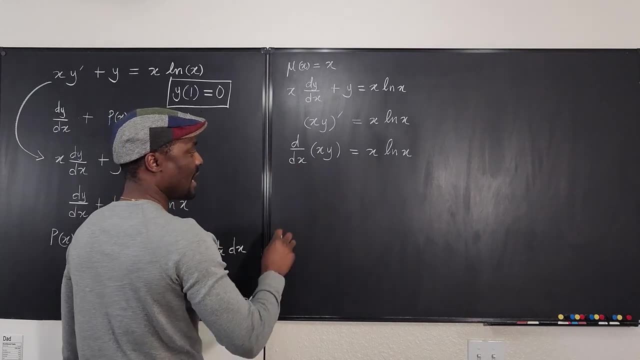 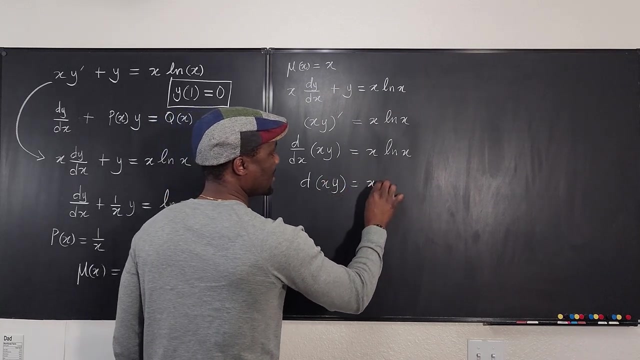 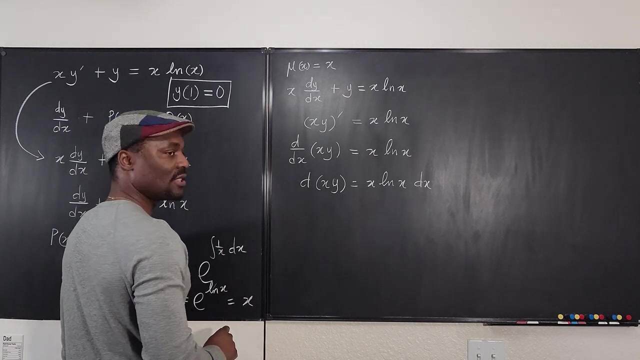 Which another way of writing this- equals x times the natural log of x. You know what we could do. We can multiply both sides by DX, so that what we have is just d, x, y equals x, ln, x, DX. Now we can take the integral of both sides. so if I integrate this, I integrate this. 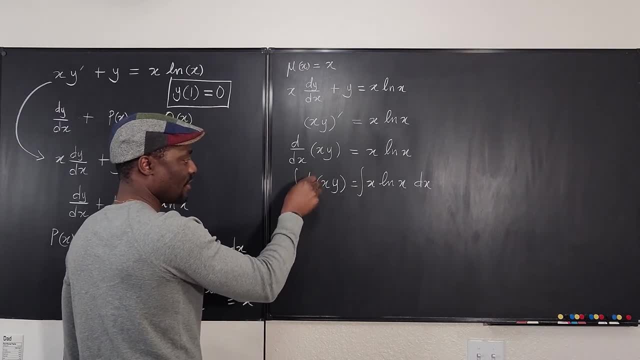 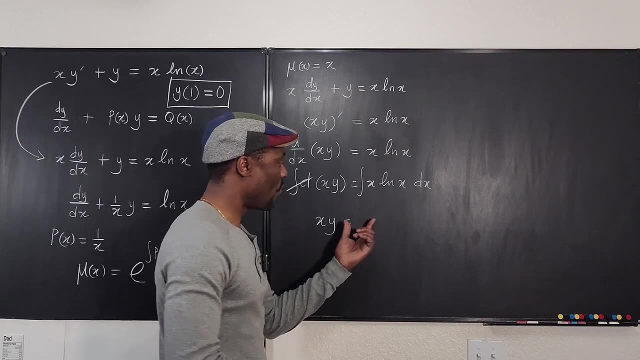 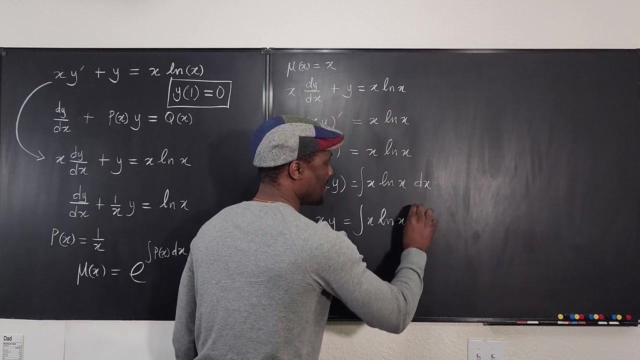 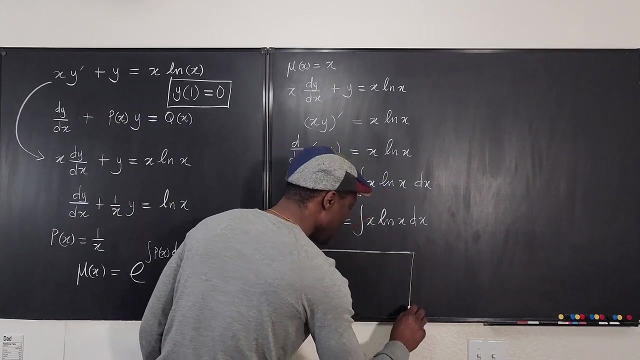 See this integral sign will take out this d. That's how you you should view it, so that what is left is just XY equals the integral of this. now, what is this integral? let's write it out: X, natural log of X, DX you'll have to use what? would you use? integration by parts? so I'm going to say that I'll 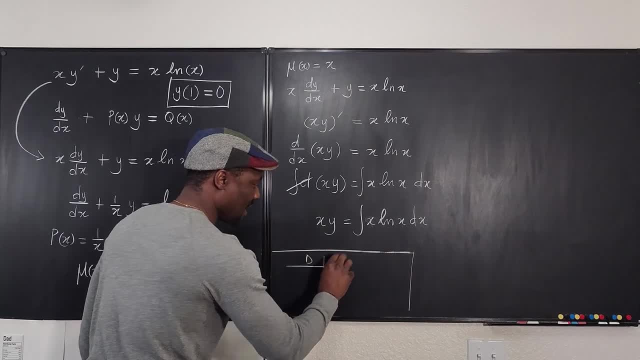 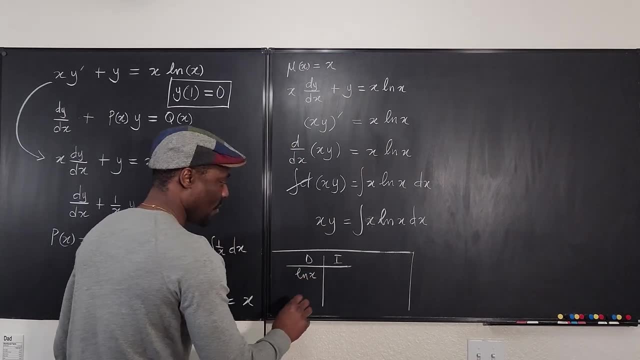 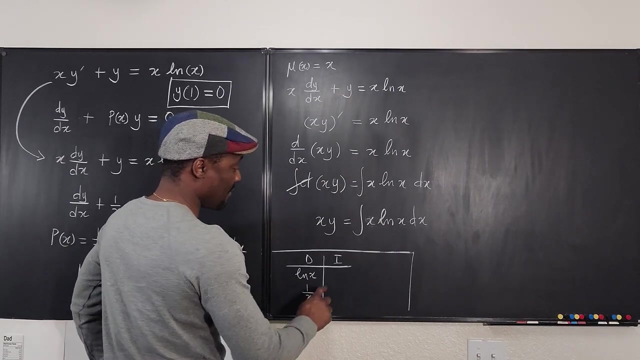 make. I'll differentiate this. so this is what I will differentiate. I will integrate this because this is easier to differentiate. so if I differentiate natural log of X, what would I get? I'm going to get 1 over X. if I integrate the natural log of X, I mean, if I integrate X, what do I get? I get x squared over 2. okay, 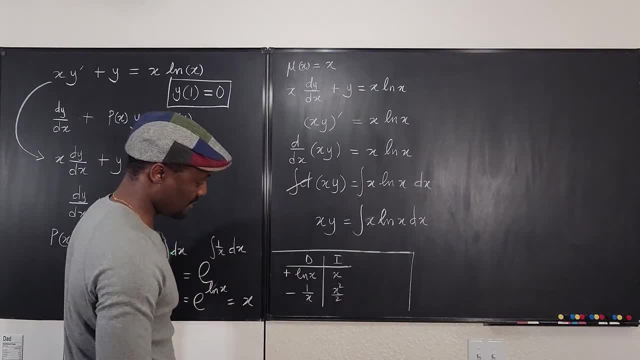 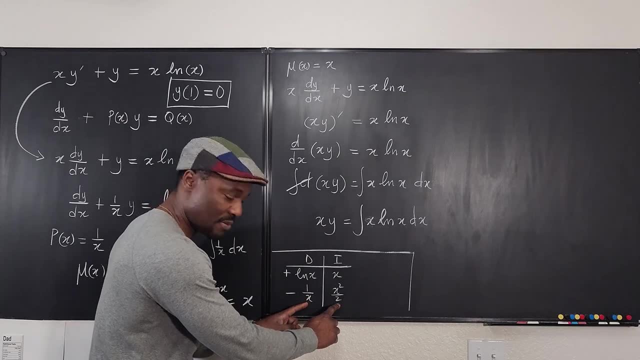 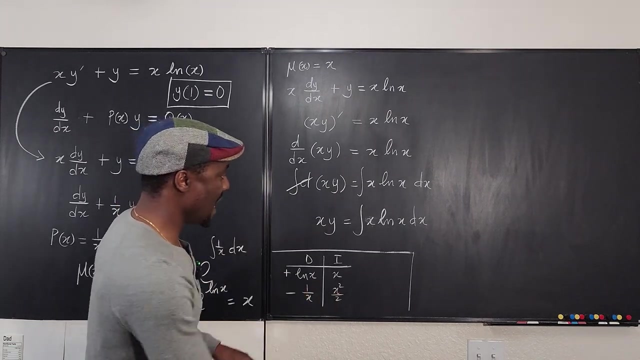 so I put the sign plus minus. you could do it anyhow, but I like doing this, and this is not going to get better. but it has gotten to a point where I have a polynomial, because if I multiply across I'm going to get just X squared over 2. so my answer to this- let's continue here so I can say that XY is: 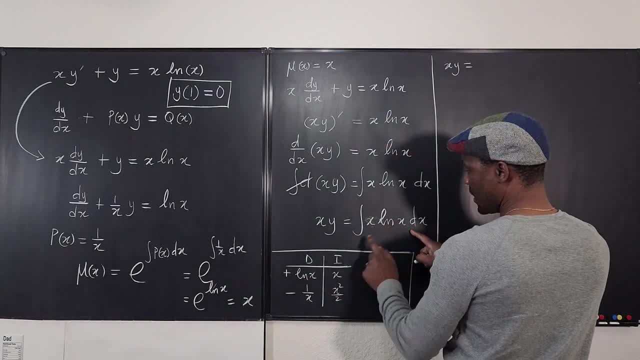 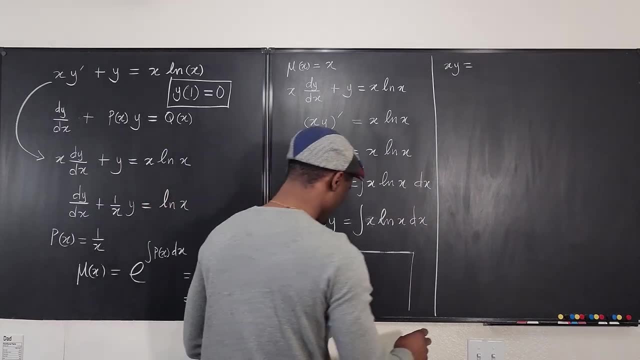 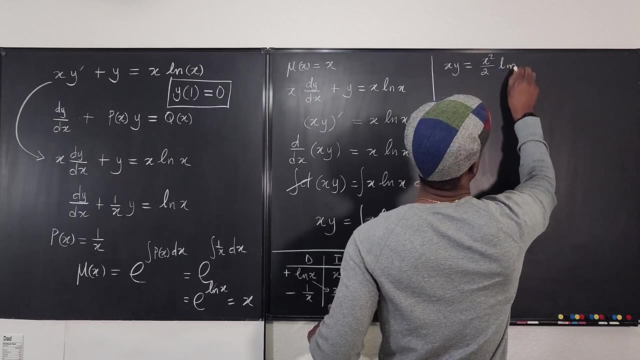 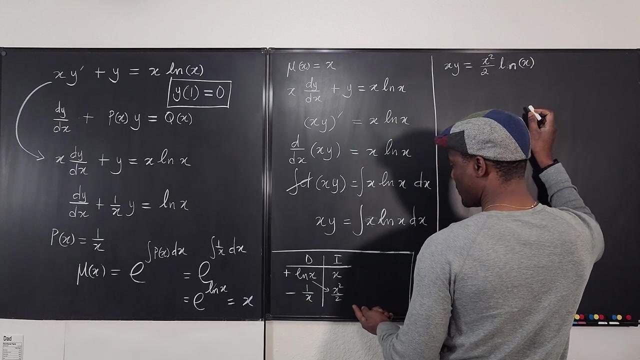 equal to this integral. this integral here can now be written as plus natural log of X times x squared over 2. so that's going to be equal to x squared over 2. natural log of X. sorry, natural log of X. and then we go to the product across. I just stop because I can integrate this. 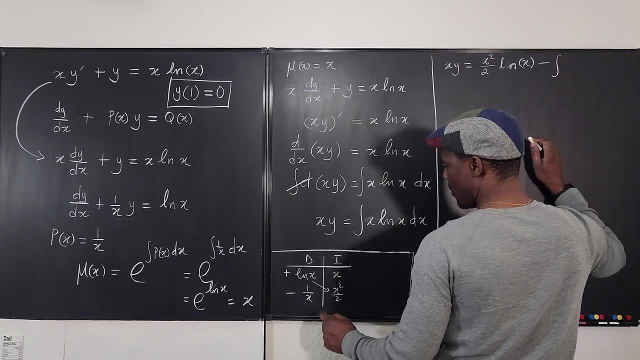 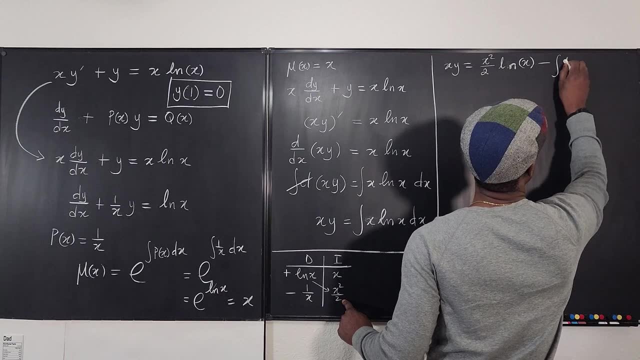 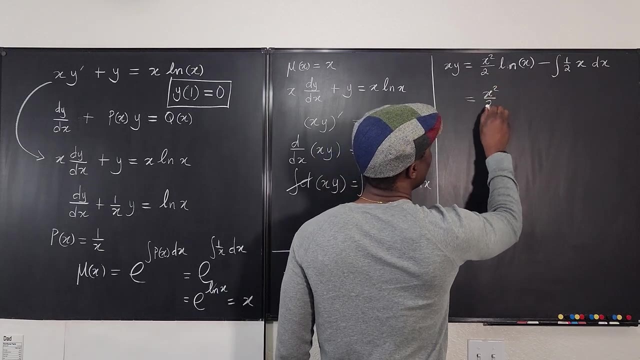 easily minus the integral of this product. what is 1 over X times x squared over 2, that's going to be half of X, so I can integrate 1 half of X. this is the same thing as x squared over 2 times natural log of X times I mean minus 1. 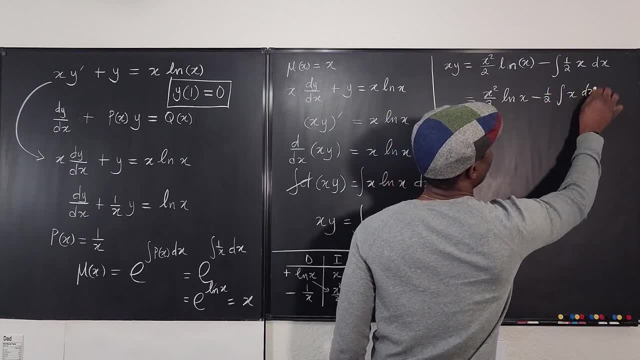 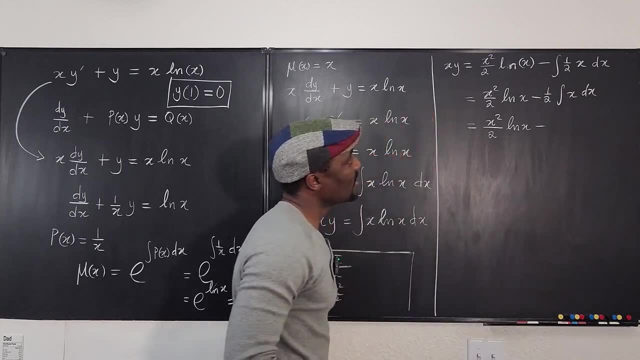 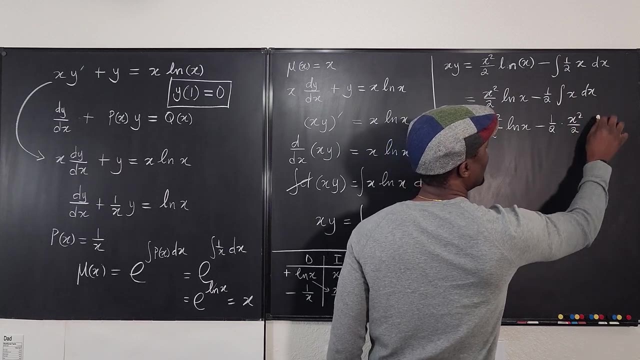 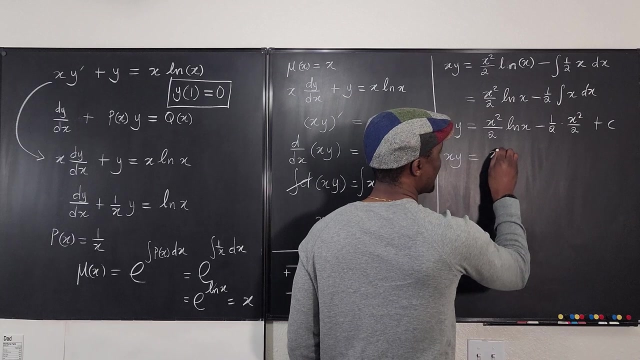 half of the integral of X dx. well, that looks like x squared over 2, natural log of X minus 1. half of the integral of this is going to be x squared over 2 plus C. we're almost there, so we have XY now. XY equals, so let's make it x squared ln. x over 2 minus x. 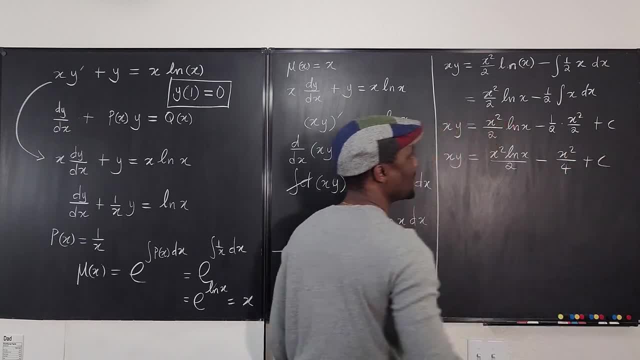 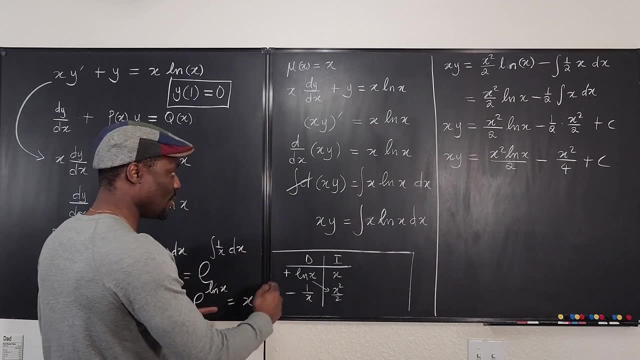 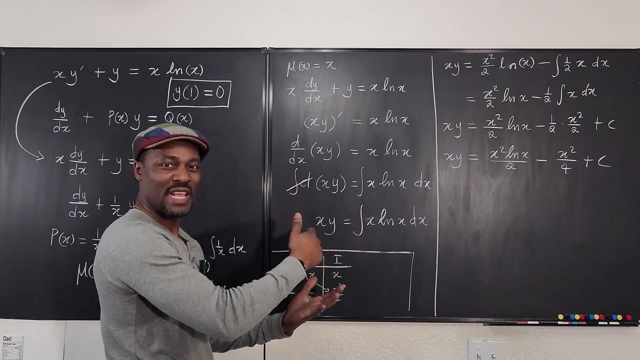 squared over 4 plus C. remember to introduce your plus C as soon as you integrate the right-hand side, as soon as you integrate this side, make sure you introduce plus C. you don't need to put a plus C on the side because, as you see, we didn't really do any. 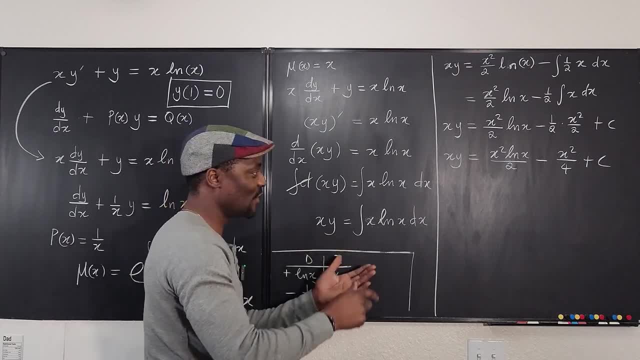 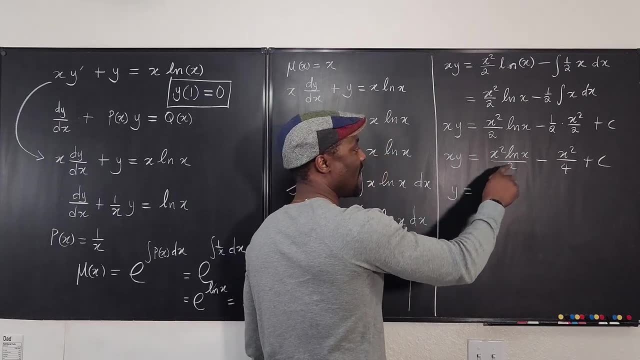 integration. we, it was just a modification, okay. so here what you want to do is isolate Y, because that's what we're looking for. so we're going to divide every term that we have by X. so here we're going to end up with X over 2.